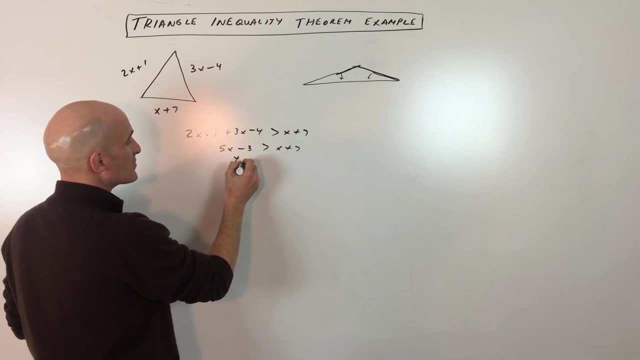 3 is greater than x plus 7.. If we subtract x from both sides, we get 4x. If we add 3 to both sides, we get 10.. And if we divide by 4,, we get x is greater than 10 fourths which. 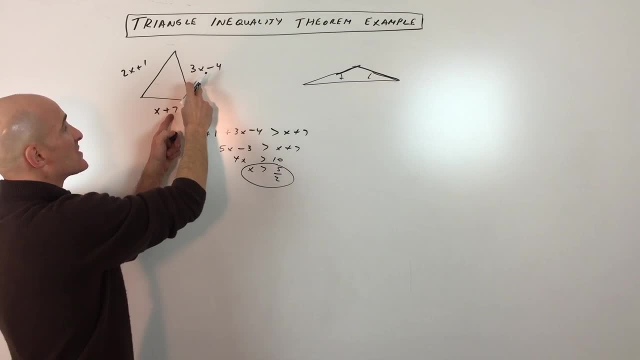 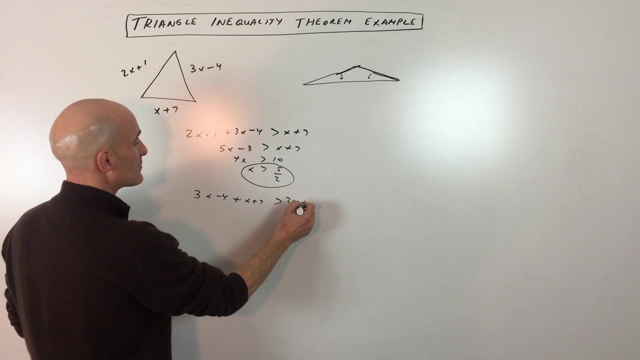 is 5 halves. Okay, now let's go ahead and use these two sides. They have to be greater than that third side. So we have 3x minus 4 plus x plus 7 has to be greater than 2x plus 1.. So this gives us 4x plus 3 is greater than 2x plus 1.. If we subtract 2x from both, 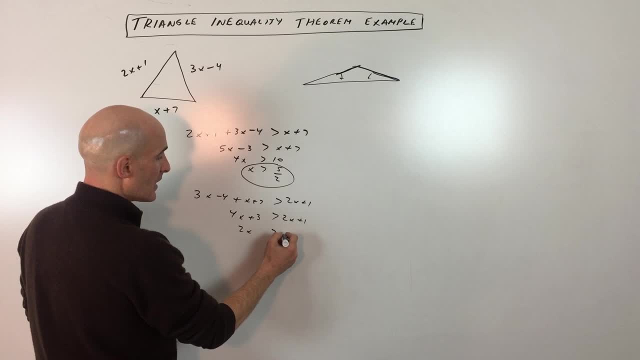 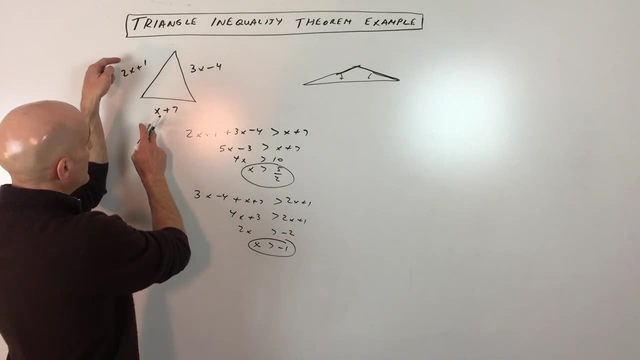 sides we get 2x. From both sides we get, let's see, negative 2.. And if we divide by 2, x has to be greater than negative 1.. Okay, and then the last one is: let's see, we've done these two. We've. 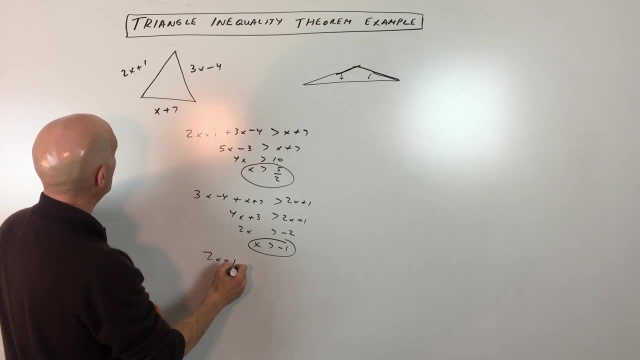 got. these two are greater than this one here. So we've got 2x plus 1 plus x plus 7 has to be greater than 3x minus 4.. Okay, so here we get: 3x plus 8 is greater than 3x minus. 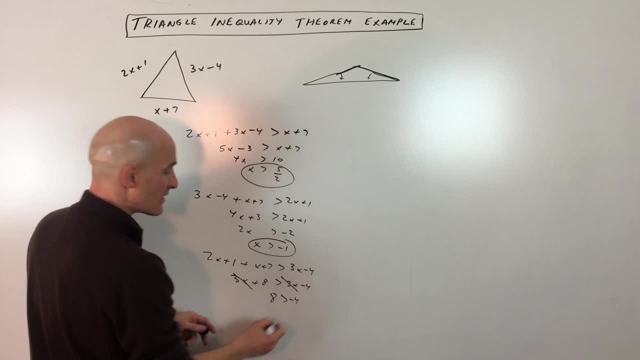 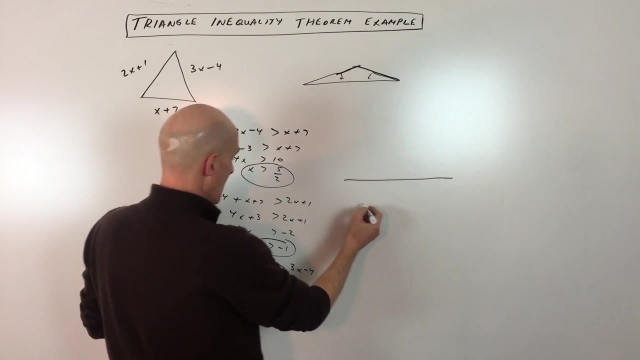 4.. And if we subtract 3x from both sides, we get 8 is greater than negative 4,, which is all always true, So we don't have to worry about that inequality. So we're just looking at these two here. Now, if we graph these on the number line, let's see here's negative 1,. 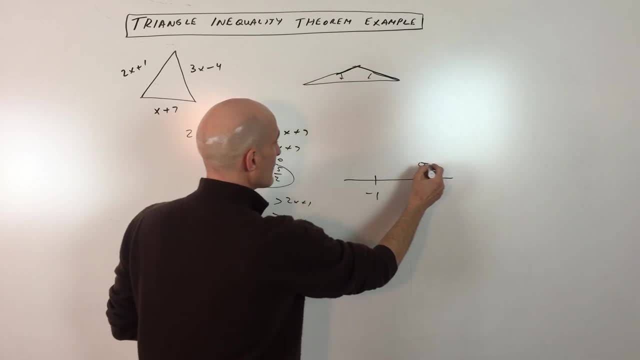 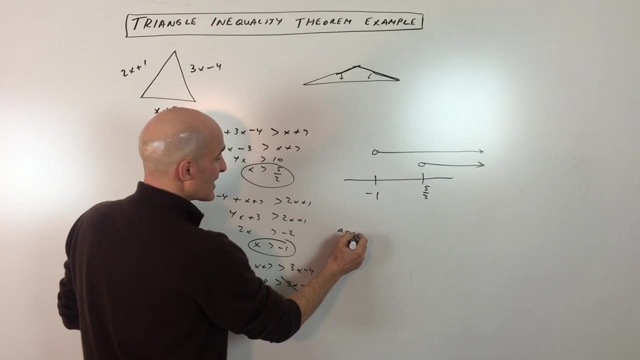 here's 5 halves, right? So if you're greater than 5 halves, okay, and you're also greater than negative 1, now when you think of the word, and it has to satisfy both of these requirements, right, It has to be greater than 5 halves and greater than negative 1.. 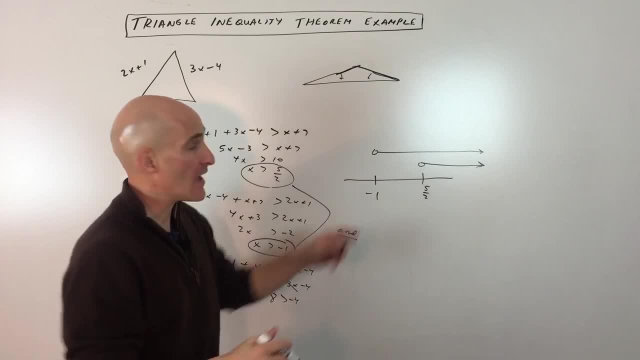 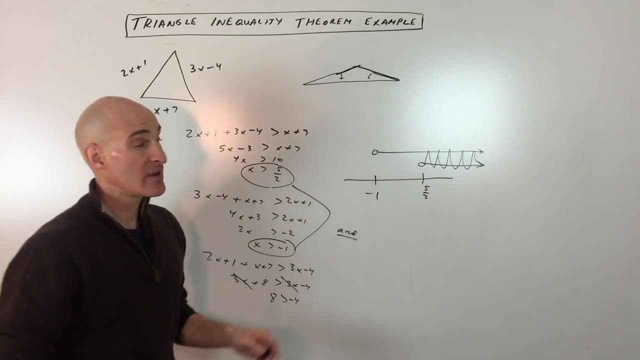 In math, you know, and means the intersection. It means the overlap of the two sets. So where do they overlap? They overlap right here. As long as you're greater than 5 halves, you will also be greater than negative 1.. But just because you're greater than negative 1 doesn't mean that you're going to satisfy. 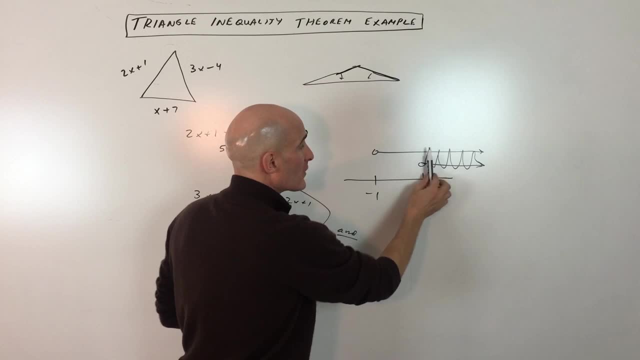 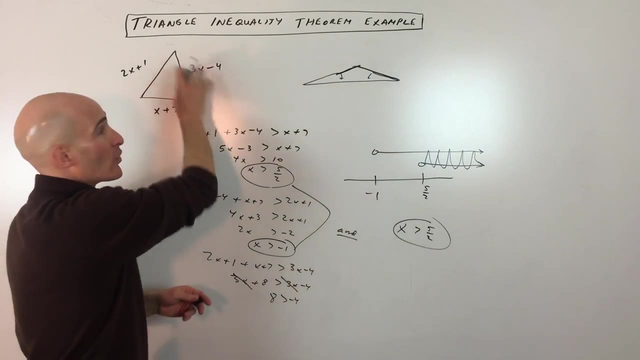 the requirement of being greater than 5 halves. So we look at where they overlap or intersect and you can see that as long as x is greater than 5 halves, then we're going to be able to form a triangle with these three sides. So I hope this helped you understand how to. 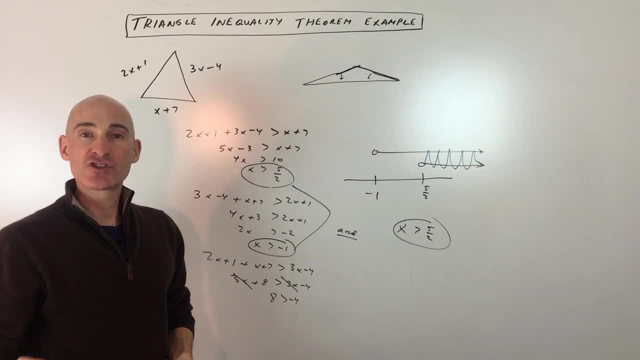 work with the triangle inequality theorem better Subscribe to the channel. check out more math videos on Mario's Math Tutoring YouTube channel and I look forward to seeing you in the future videos. I'll talk to you soon. I'll talk to you soon.